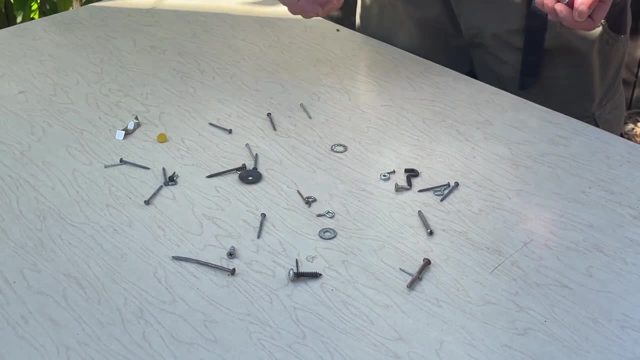 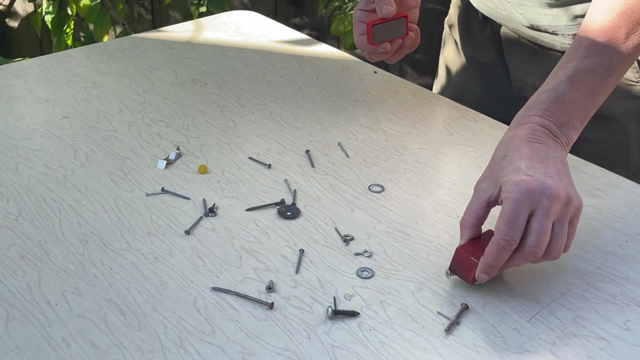 And they're all kind of spread through the soil. They're not really doing much good, They're kind of just kind of hanging out by themselves. But the beauty of humus is that when there's humus it acts like kind of a collector and it collects all of this stuff into nice clumps. 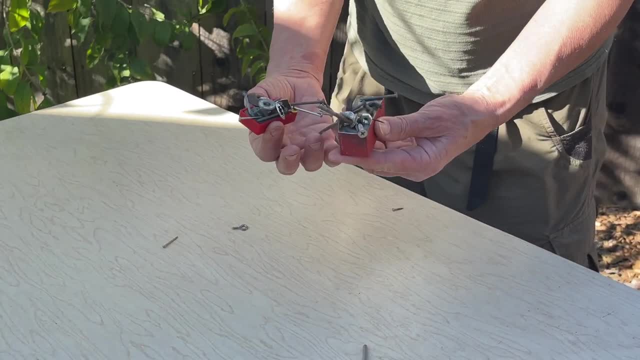 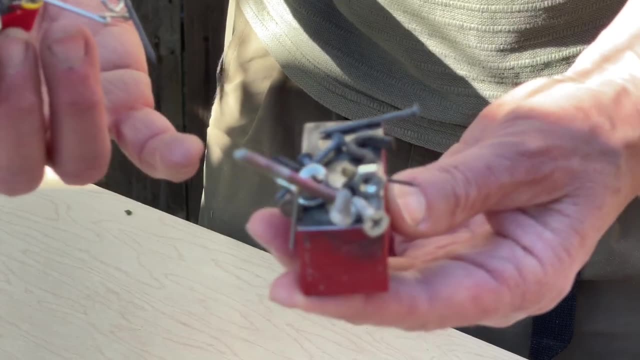 also known as aggregates, And these aggregates are very beneficial for the soil because they create big pores or air spaces that oxygen and water and the roots of plants can all kind of get through, And they're very beneficial for the soil because they create big pores or air spaces. that oxygen and water and the roots of plants can all kind of get through And they're very beneficial for the soil because they create big pores or air spaces that oxygen and water and the roots of plants use those pores to seek out the oxygen that they need and the nutrients and the water and the moisture. 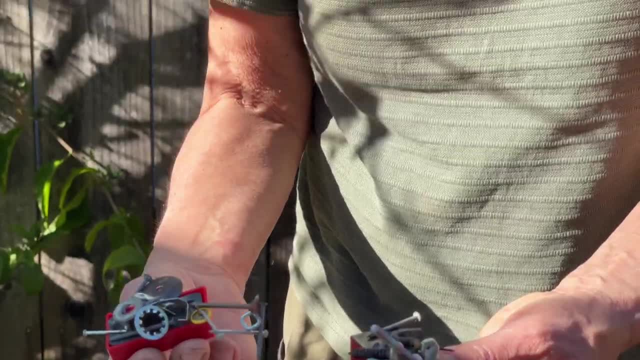 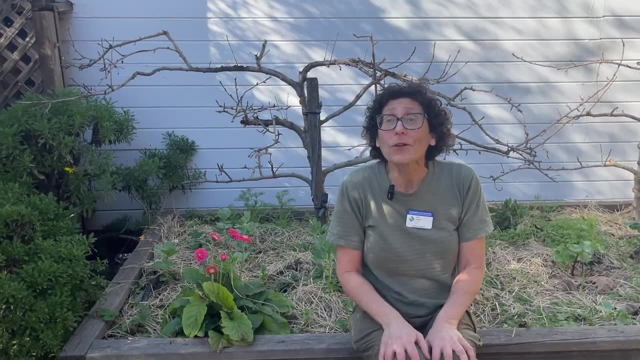 So these large aggregates are very, very beneficial, And this is what humus does for us in soil. So these large aggregates are very, very beneficial, And this is what humus does for us in soil. Okay, so aggregates, Why are they important? Well, humus is very important because it stores a lot of the carbon. 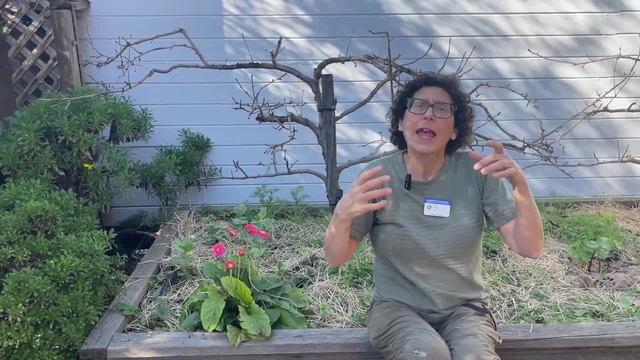 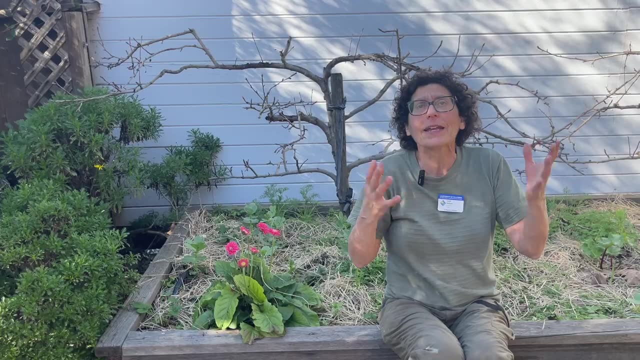 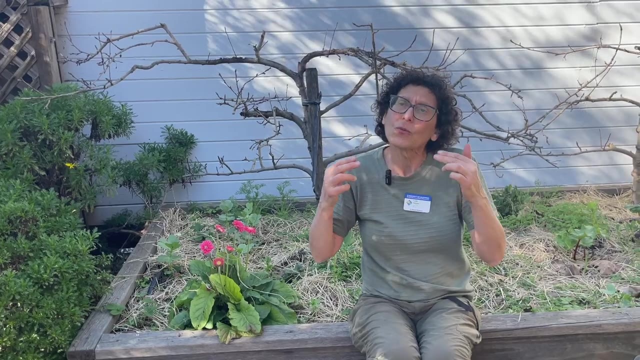 that's released into the atmosphere by the burning of fossil fuels, And it makes it possible for the soil to just kind kind of hold it there safely without contributing to this blanket effect that's warming the earth. But humus does a lot of other really important things too. It slows the release of water, so that 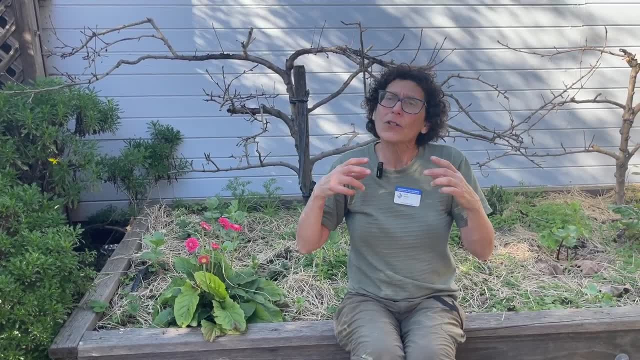 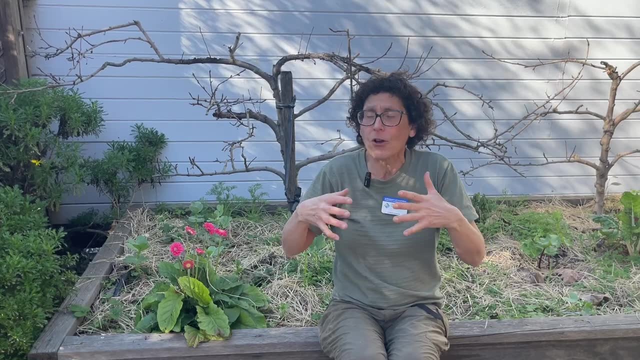 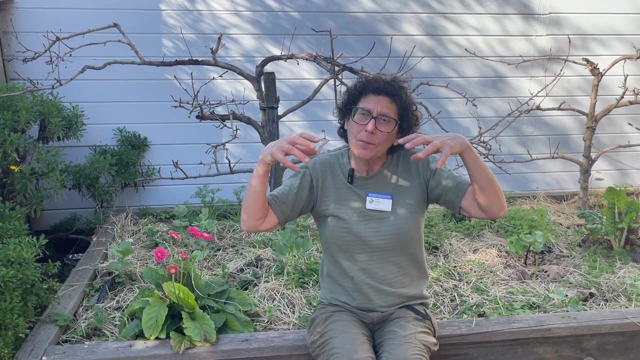 plants can get the amount that they need appropriately, and it also allows the minerals to be taken up by the plants at the right pace. It's called mineralization, so that the plants are getting the nutrients that they need from the soil, and it allows the pores to be a space where 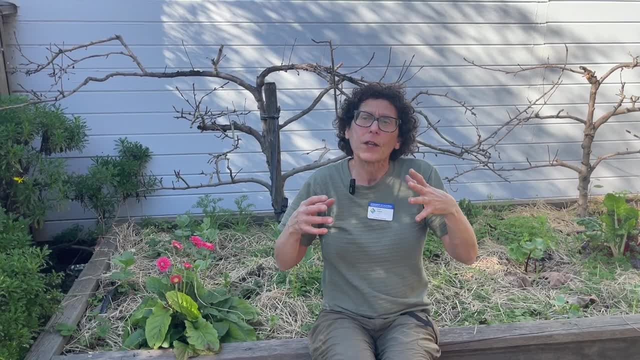 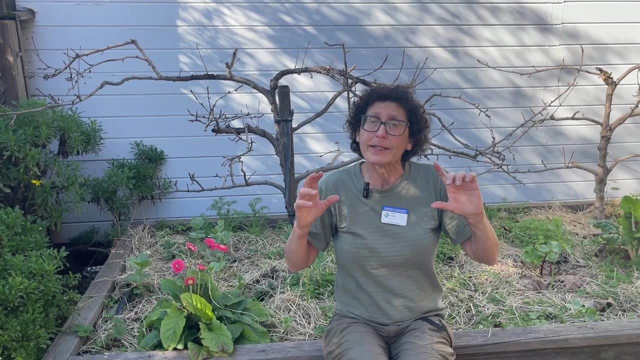 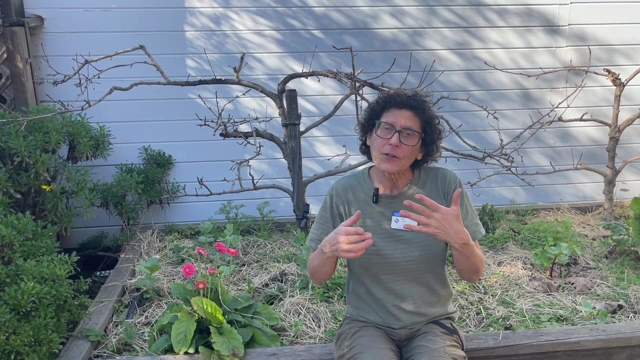 the roots can come and look for those things that they need. So humus is very important in supporting root growth. It also can increase food security because it makes it easier to grow food by doing all these things that I've just described, and it does some things that are good for the 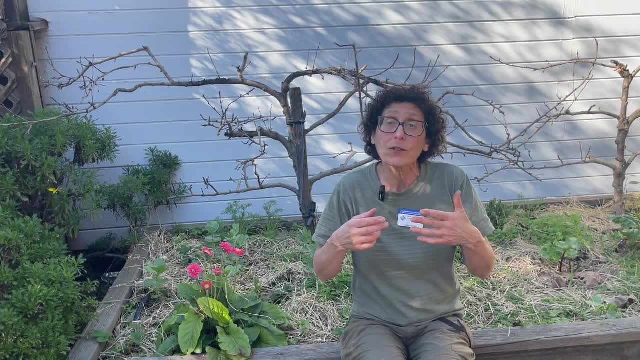 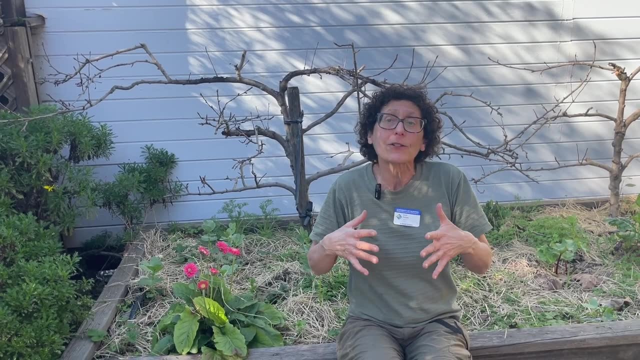 environment too. It buffers the pH of the soil, so it's not too acidic. It's not too acidic and not too basic. It kind of creates that middle zone. It binds heavy metals and it filters water pollution. So humus is something that we all really want and need in our gardens.